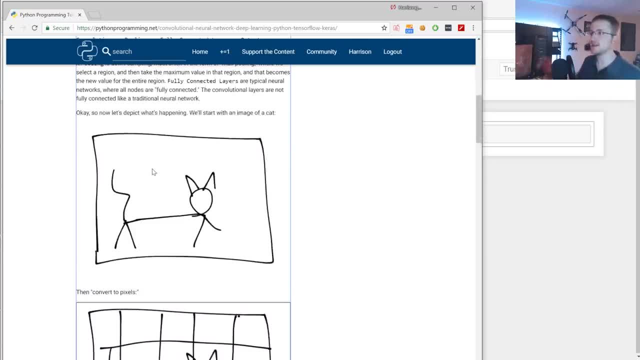 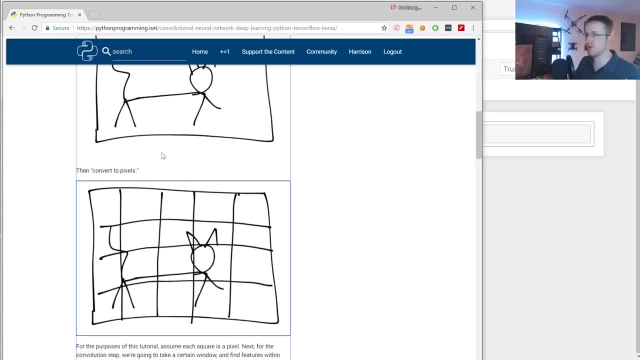 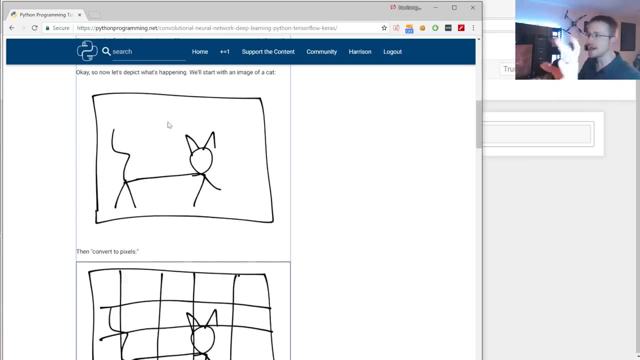 So let's talk about that. So first of all, the idea is convolution is defined, you know some sort of useful thing, and then we pool these useful things together for the combination of convolution and pooling for your convolutional neural network. So the idea of this is like, let's say, you take an image and then we convert that image to pixel data. So 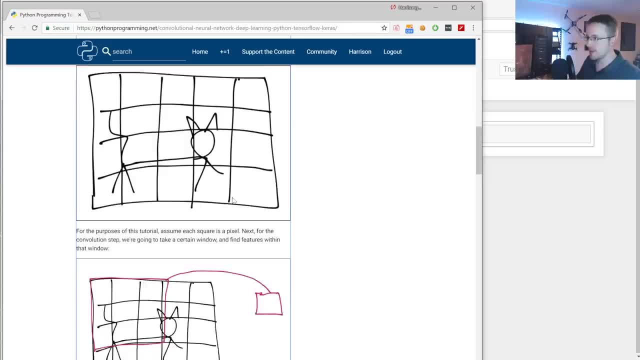 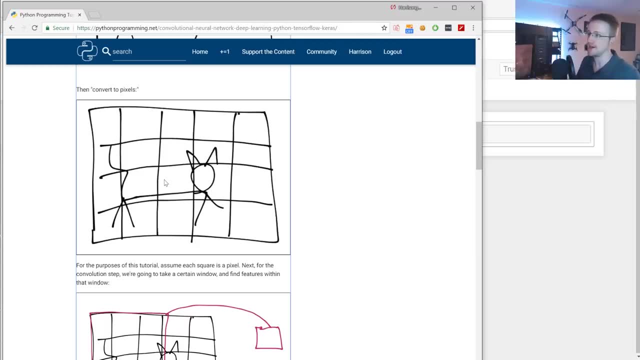 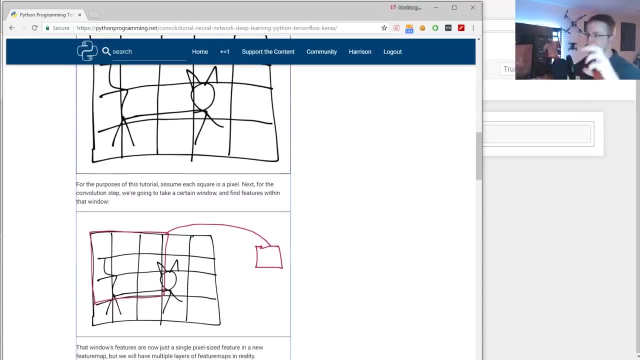 this is just my- you know bad representation of pixels, But anyways, you convert to grid or after it's been converted, to pixels. like this in theory could be a convolution on top of a already. you know there's already been a few convolution Layers, but anyways, the idea is, then you have a window like a convolutional window, in this case. 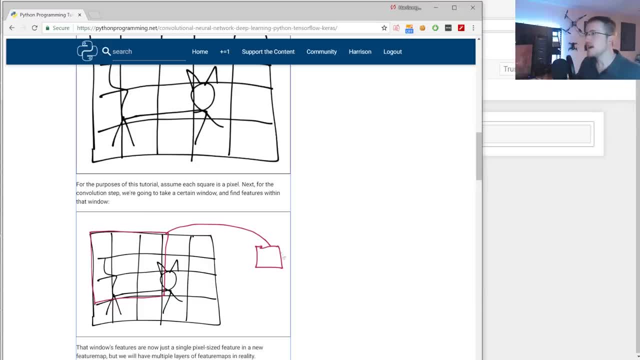 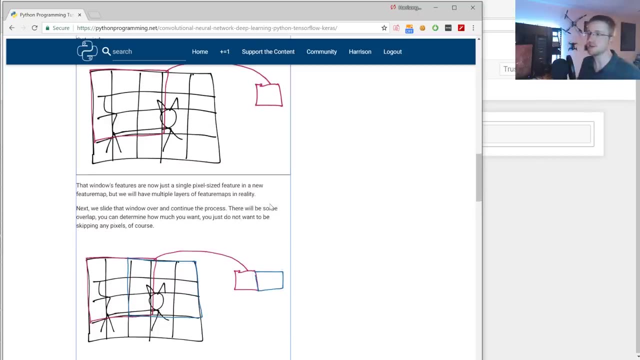 it's a three by three window and in that window the convolution is going to attempt to simplify what it finds down to some sort of value. Now, when it does that, the window is going to shift over and do the exact same thing just a bunch of times. So, in general, you've got the window, you've got how. 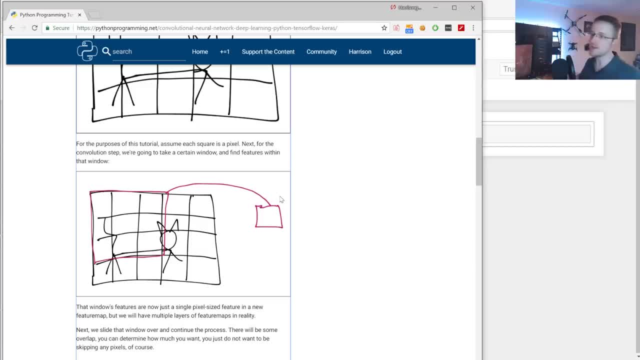 big of a stride over do you want to take, and so on. Now, with Keras, you've got the window, you've got. you can really just specify the window size and that's it. And like everything else, like someone was asking in the previous, well, the first video about bias. If you want to learn more about the 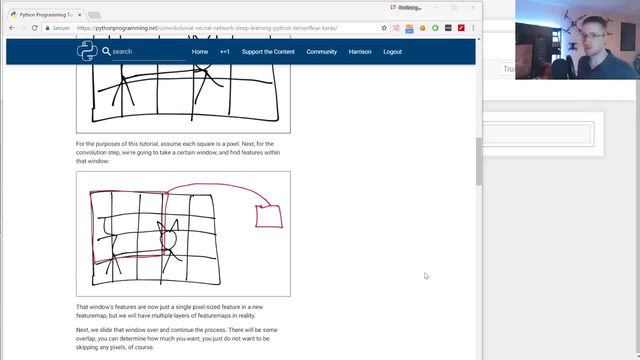 more deeper details of deep learning, go to the practical machine learning tutorial series where everything is much more deeply explained. because it has to be deeply explained because the way we were writing that was with raw TensorFlow code. So definitely go check that out if you want to see more of the inner workings and how things are done, Like, for example, if you're 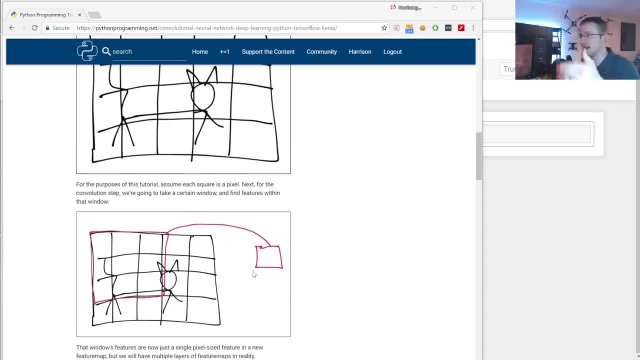 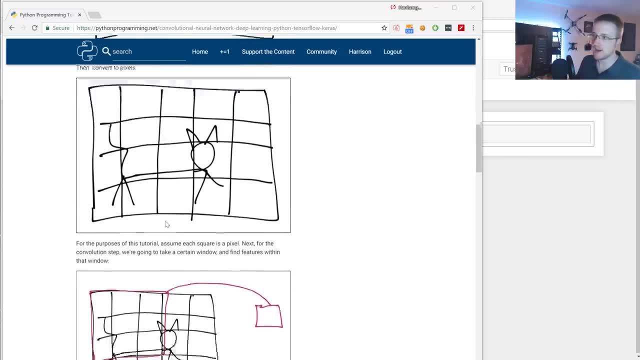 going to do a simple: as you keep sliding, what happens when you slide over the edge, You know most cases we're probably going to pad it. but then do you want to pad it like, or same, or all this stuff? So anyways, getting back to what we're doing here, So it'll produce features, so in general, and then 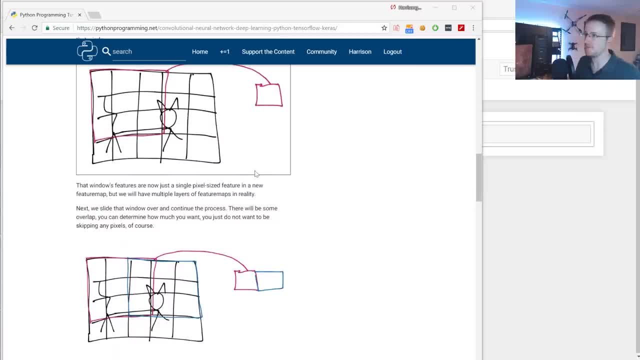 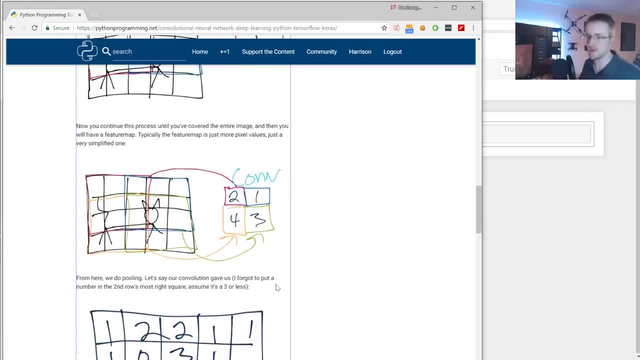 you'll do it many, many times. So it's a way to kind of slowly extract features from an image. So convolution, convolution, and let's say the convolution produces a two, a one, a four and a three. Now, these aren't. it's not going to look just like that, but just for simplicity's sake, 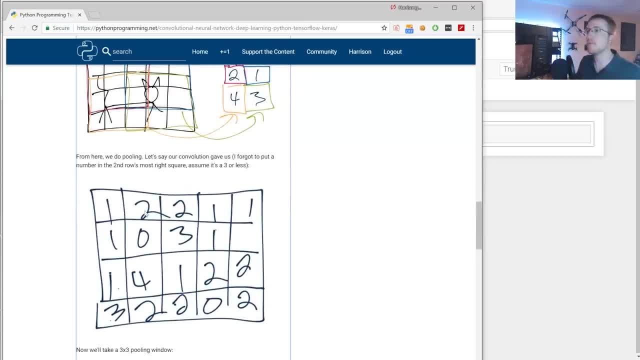 Let's say it's a two, one, four, three. Then let's say: you've got a bunch of convolutions. Right, This is just a bunch. The next thing that's going to likely happen- you don't have to, But this is pretty common- is to do a pooling layer. So, in general, the most common form of pooling is max pooling. 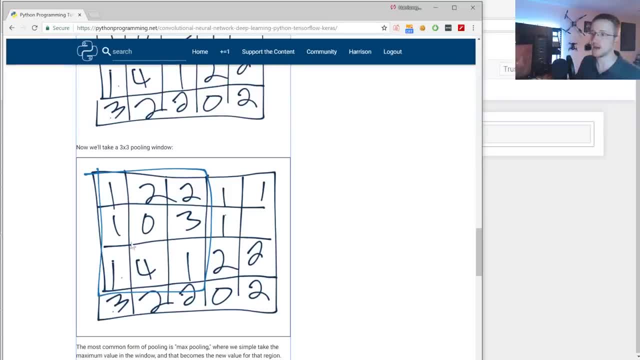 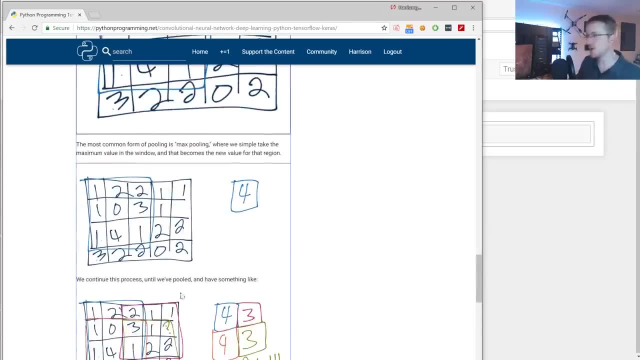 So again, let's say you do a max pooling of a three by three window. Well, all max pooling does is find the max value. So in this window the maximum value it's a four. then it shifts it over and again and again. So you can see how it, how it worked, basically down here. 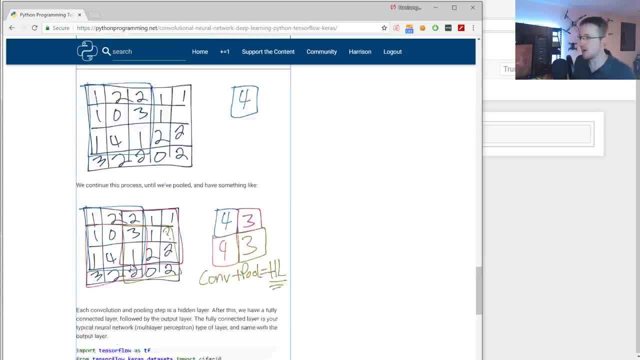 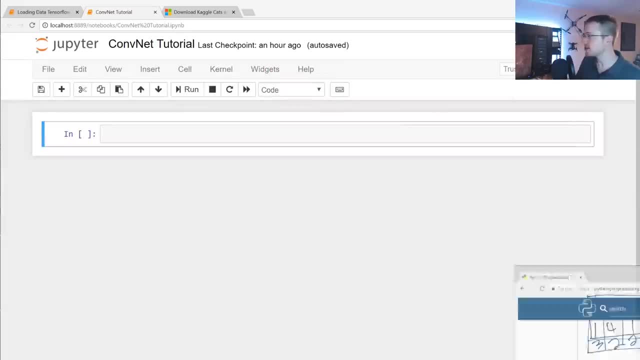 So that's convolution and max pooling. Now the higher level idea of how this actually works is basically it's slowly extracting value from the image. So, lower the more, initial layers in a convolutional neural network are going to be finding things like edges and lines And then, as you go, you're going to find like maybe. 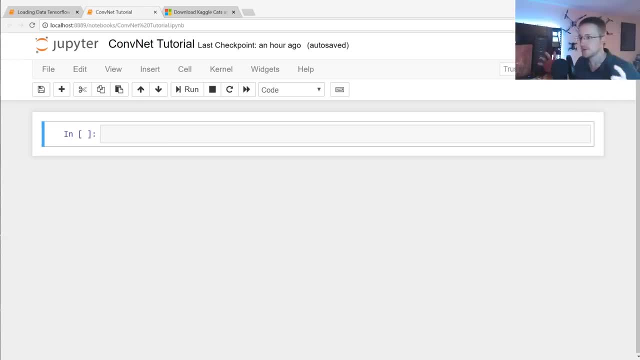 maybe squiggles, and then maybe you'll find circles, and then maybe you'll find squares, And then soon you're going to find, I don't know, like very small, like features. So, for example, if you're curious- I don't know if this is going to play some sound- It is. 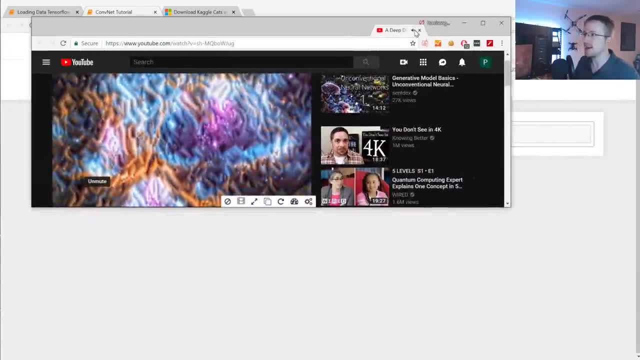 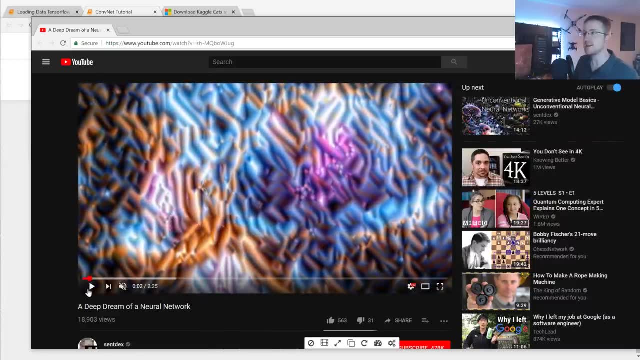 Let me just mute it. This was a deep dream And what you can see actually going through this is how what a convolutional neural network is, kind of basically a deep dream, is going to accentuate what it finds. So these are the initial layers, where it just finds a bunch of straight lines. 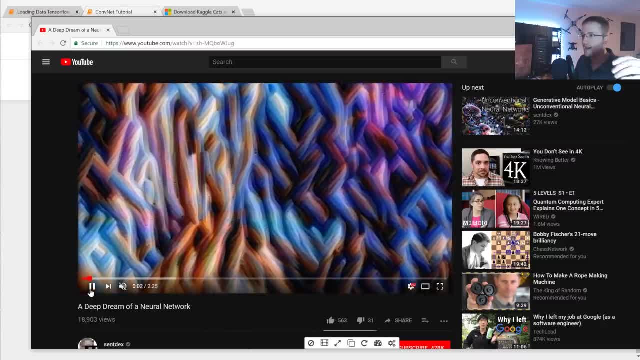 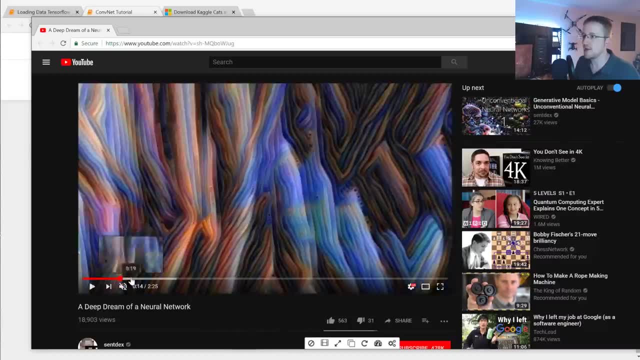 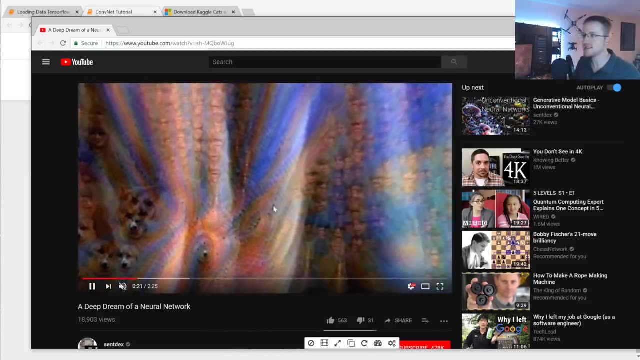 And then as you go a little little deeper, you start finding slight curvatures and lines and then as you continue on, you'll find, hopefully, something different. Yeah, it's like you get kind of more square shapes right, And then as you continue along we start getting like faces and eyes stuff like that. as we continue even further, you start getting it like you can almost recognize a dog there. 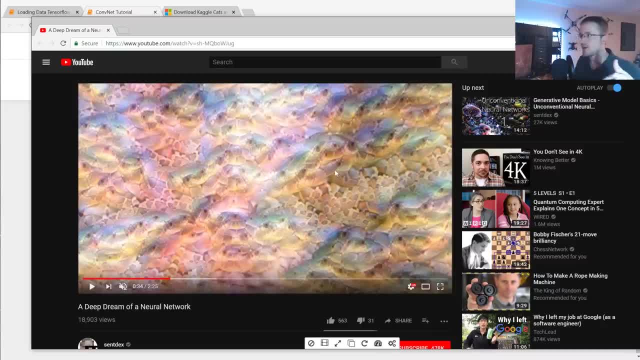 And then as you get closer, you start getting like even bigger lines. So this is the further and further in the network you start seeing things like scales and stuff like this was trained on um, like uh, what was it? pet, not pets- i'm trying to think of the term um, but this: 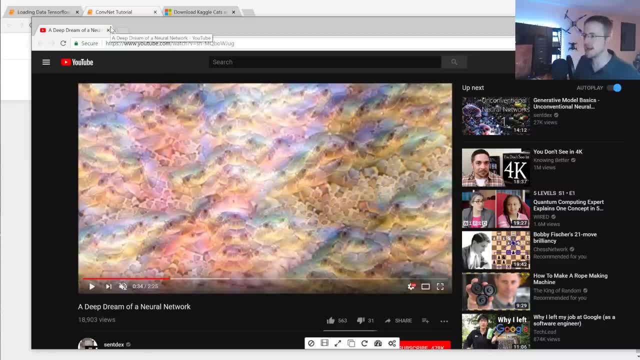 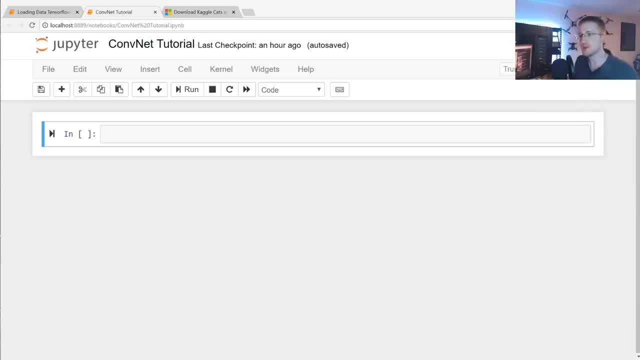 was off of. i'm trying to think it was the image, i think it was the image net data set. anyways, this was inception off of the image net data set. but anyway, you can check out a deep dream of a neural network. if you want. also you could check out the- uh, that series, the unconventional neural network. 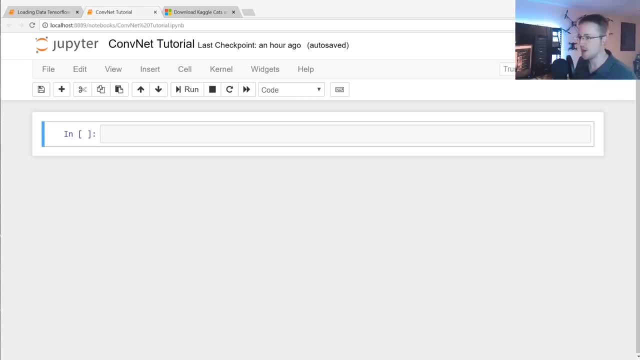 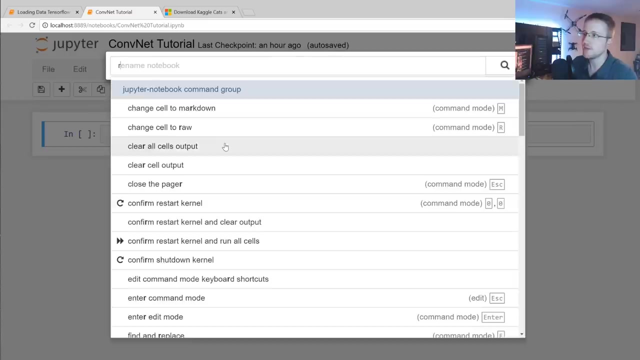 series, uh for more on, uh, more interesting projects like that. so okay, so the first thing that we want to do uh is bring in um tensorflow and all the things that we need to make a convolutional neural network. so we're going to in, not do that, we're going to uh import tensorflow. 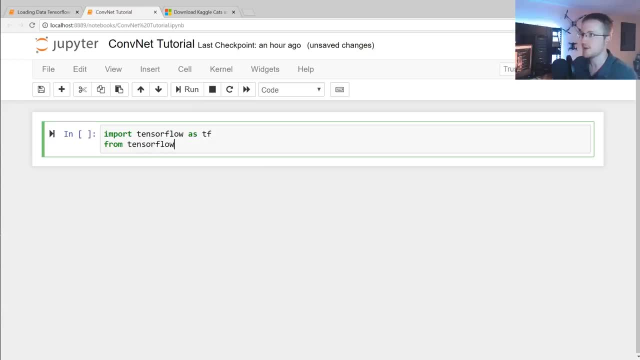 as tf. we're going to say: from tensorflowkerosdatasets. um, actually we don't need to import any data sets, just kidding. uh, what we're going to do first is bring in um from tensorflowkerosmodels. we're going to import sequential because we're going 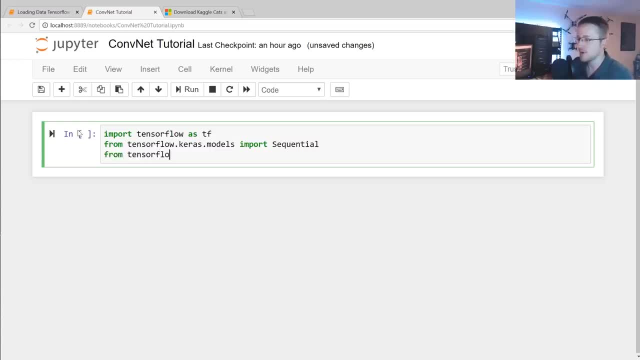 to use that sequential model. then from tensorflowkeroslayers we're going to import dense, so your typical dense layer um. we're going to import dropout, we're going to import activation um, and so first of all we're going to import the um, the dense layer, because a lot of times you're going to end um either a recurrent net or a conv. 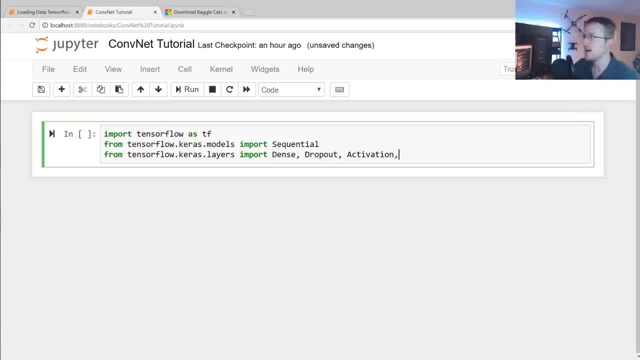 net with a final dense- uh, just fully connected layer and then also flatten, and we're going to use flatten before we feed it through that final dense layer. then we also want to bring in conv 2d, capital d and then max pooling 2d. okay, so then we're going to import. 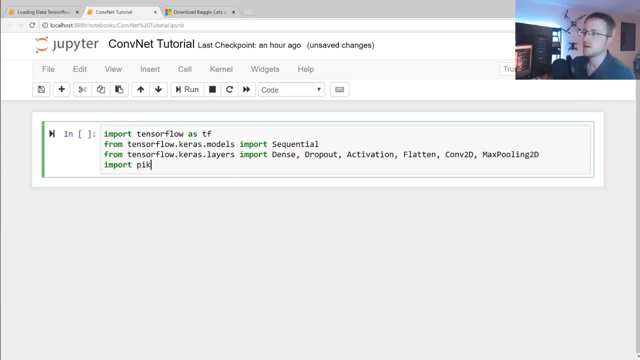 import pickle pickle and we're going to do that, uh, pickle, or actually we can just do this: we can say x equals pickle, dot load, and we'll load in open x dot, pickle, pickle rb, and then we'll do the same thing for y. so x, x and y. so then, the first thing we want to do before we feed data through a neural network, 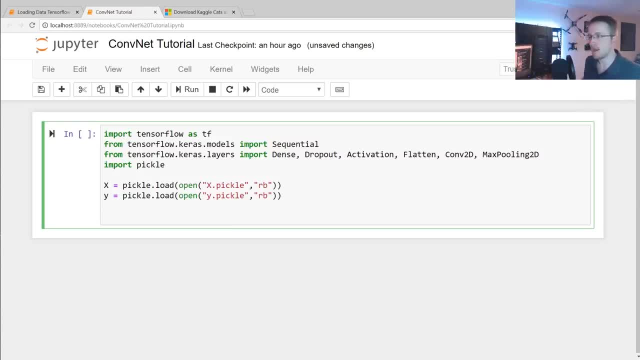 is consider normalizing that data. the easiest way to normalize data is going to be to scale that data. in our case, we're using imagery data, so actually the easiest way to scale the imagery data is we know what the maximum value and the min value is. the min is zero. the max is 255 for. 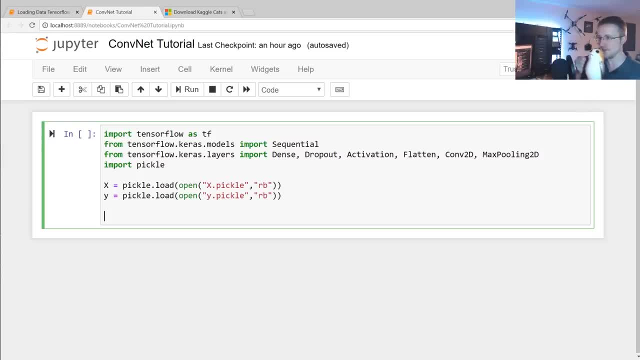 pixel data, so we can actually normalize that data by normalizing that data and then we can actually just do that. divided by 255. i need more t um, so, but there is- i think it's kerasutilsnormalize, i think it is anyways- um. in many cases you're going to need something more like that, but for now we can actually just do x. 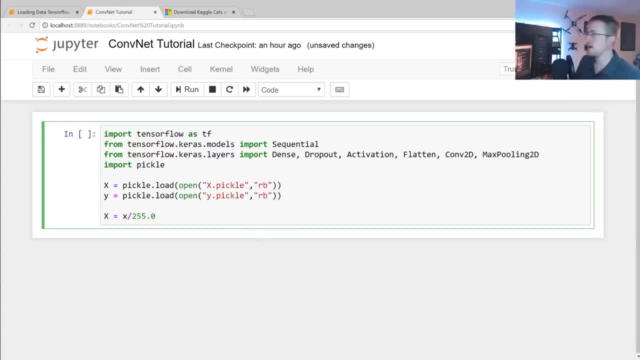 equals x divided by 255. uh, then once we've done that um, we can come down and begin building our model. so we'll start with uh, not a capital m model equals sequential, because it's just going to be a simple sequential model, and then we're going to start using that modeladd syntax that. 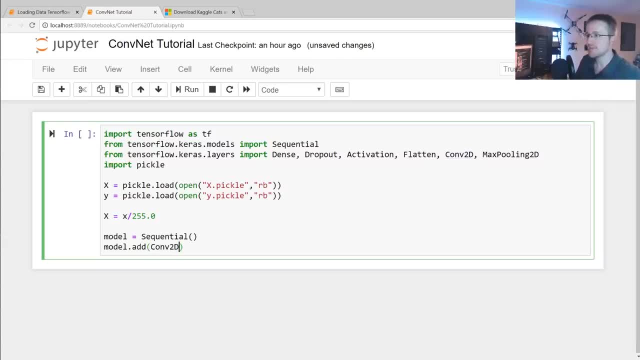 we've been using. so we're going to say conv 2d, so we're going to start with that convolutional layer, and this can be um, we can probably, we're probably- going to get away with almost anything we pass here. i'm going to pass 64, though, and then we're going to pass the window that we want to use, uh. 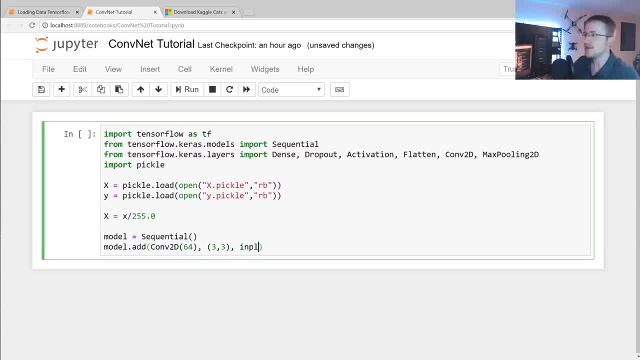 three by three, and then finally the input underscore shape is going to be equal to the x dot shape, and then here you can just say one colon, so we're going to skip that first, like negative one, so each, because negative one again is: was how many of those feature sets did we have? 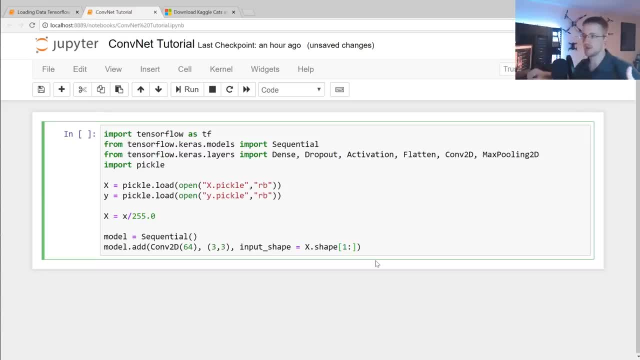 right. so we don't need that, because that's not actually the input shape. it's going to be the shape of the data we're actually throwing in, so it's not negative one, but it is, you know, 50 by 50 by 1, that's true. so that's going to be the shape of the data we're actually throwing in, so it's not. 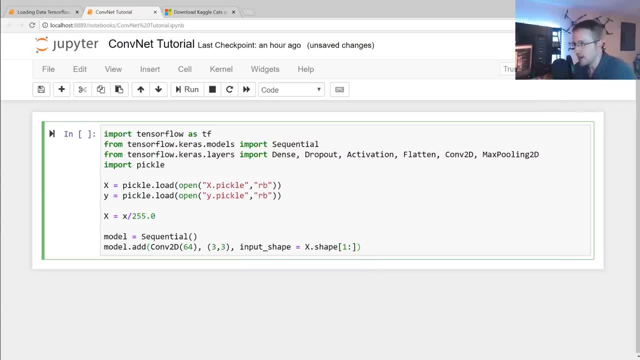 is how we can get that input shape really dynamically. so, uh, once we've done that, uh, the next thing that we're gonna do is: uh, i feel like we shouldn't be okay, whatever. uh, the next thing we're gonna do is modeladd, and we're gonna add um. 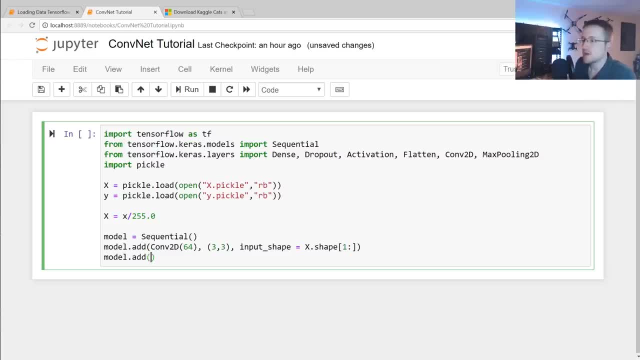 so in this case you so the, the, the max pooling again to have. so in general, convolutional and max pooling are going to go together. so in this case what we could say is, after the convolutional layer we could pass either an activation or a pooling. i'm going to go with, we're going to just do an. 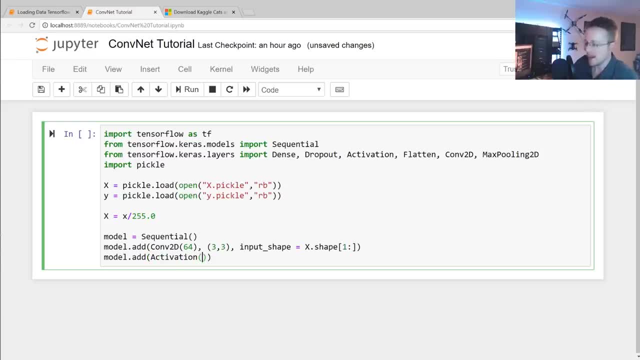 activation layer. so activation, and the activation we'll go with here is just the same one that we've been using, which is rectified linear. then we're going to do the pooling. so modeladd, uh well, i'm just going to copy this, actually copy paste: max pooling 2d, and then again here you're going to specify the pool size and 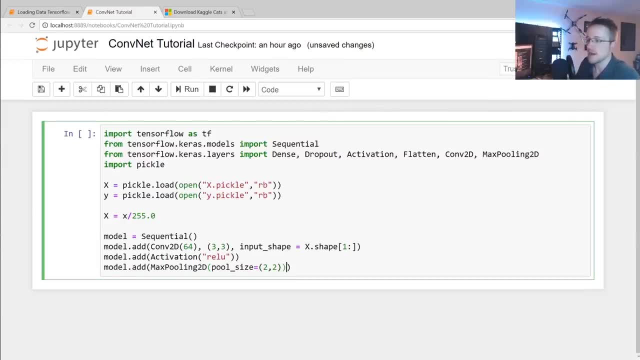 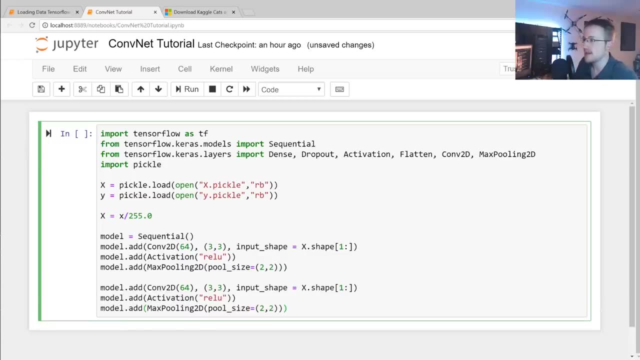 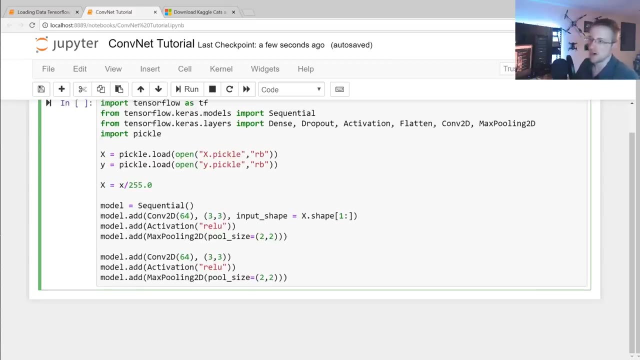 let's just do a two by two, okay, so that's our first sort of layer. now, uh, we can do this again, and this time we don't need an input shape. so now we've got a 2 by 64 layer convolutional neural network and then, like i said before, we're 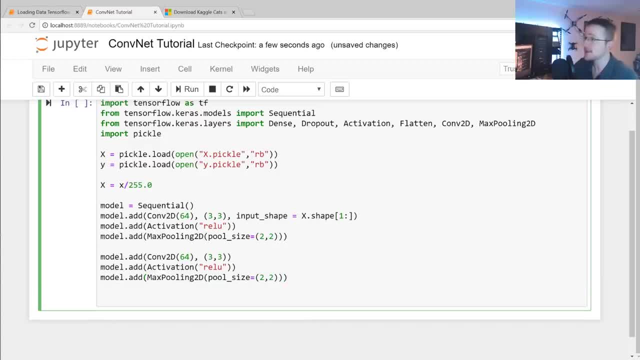 going to pass a final um. you don't have to do this again. we probably don't even need it for this data set, but just for good measure. modeladd will add a final dense layer and that's going to be a 64 node. now, before you do that, you have to flatten the data, because convolutional is 2d. 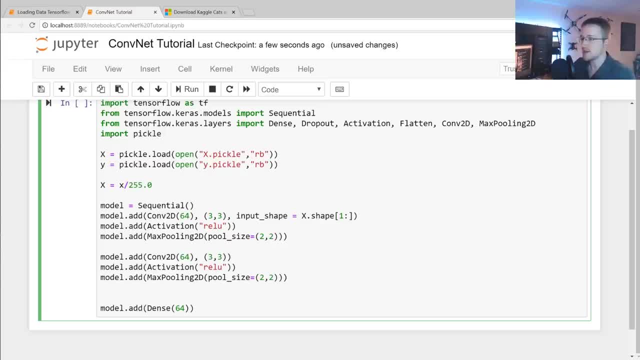 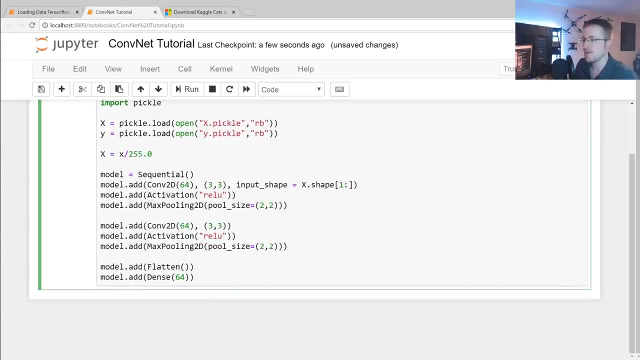 whereas that dense layer again wants a 1d data set. so we're going to say modeladd and then we just throw in a flatten. don't forget, whenever you want to do stuff like this, you do have to import that layer. um, but uh, flatten, dense64, cool. so then now all we need is that output layer, so modeladd. 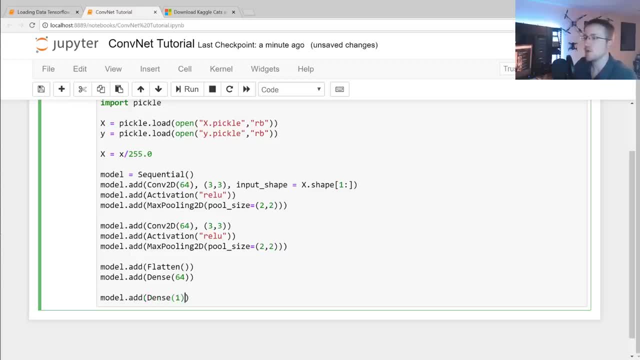 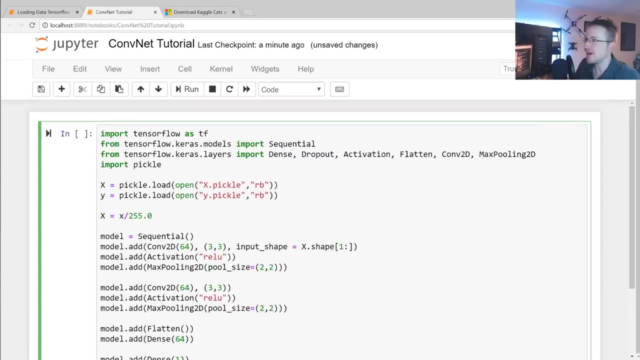 and we'll add a dense and we'll go with one and then we need that activation layer or the activation layer or the activation for it add. i feel so silly calling that a layer, but it is coming from the layers. um, i'm kind of surprised that we would call activation, for example, a layer. 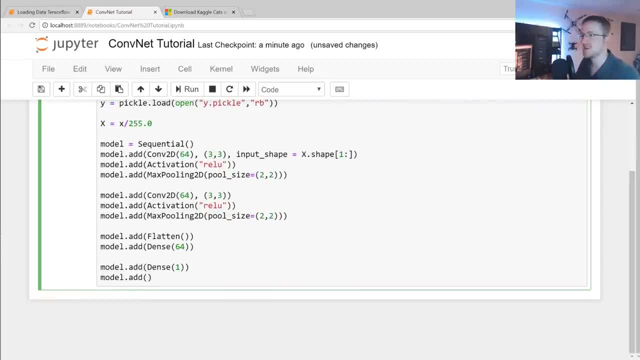 but um, okay, that's what we're doing. so anyways, modeladd and then activation. i mean, i guess it's one more thing, but in the in the old ways of doing things like you would, because you could also say dense. so like here you could say dense one, and then you can actually pass activation. 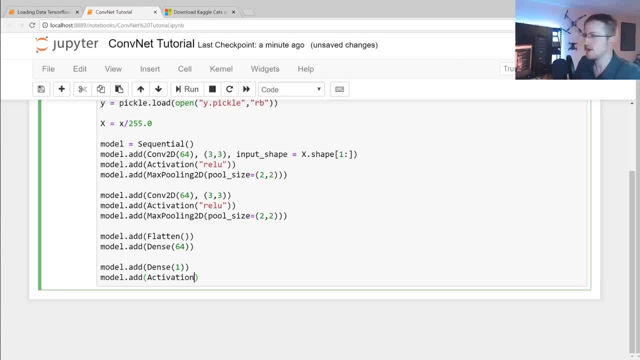 equals something. so there's a kind of like two ways to do it. so i'm not really sure why they have that in layers. but anyways, activation, um, someone could correct me if i'm wrong, but i i don't really think like i think, if you start, if you walked around calling the activation. 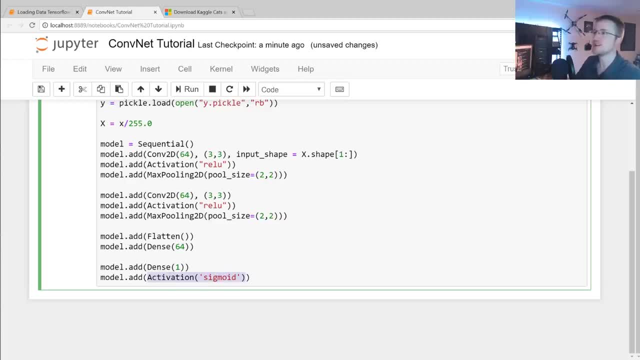 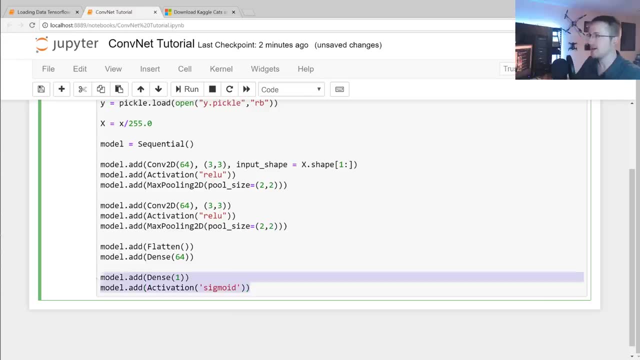 function, a layer in a neural network, like if you consider this neural network to not. you know, when i look at this i see one layer, two layers, Three layer, and then like the output layer. so really I would say this is three layers, But if you started calling this a one, two, three, four, five, six, seven, 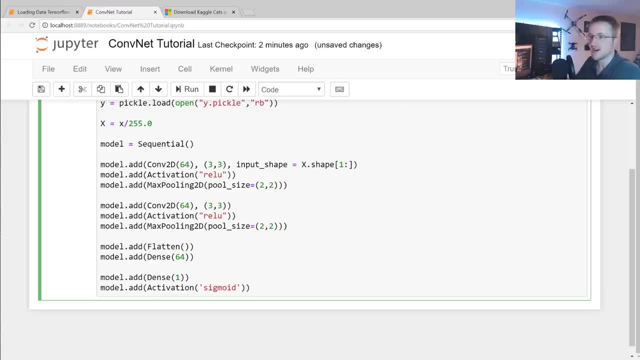 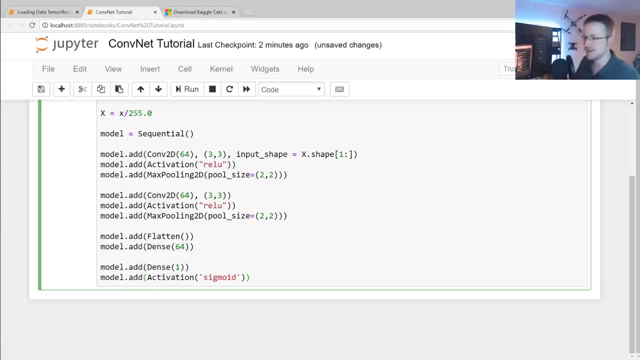 eight, Nine, ten layer confident. I think most people would disagree, but I don't know. they're throwing that in layers, So I don't know if that kind of opinion has changed in the ml community or what. anyways, model dot compile and then we'll do loss. 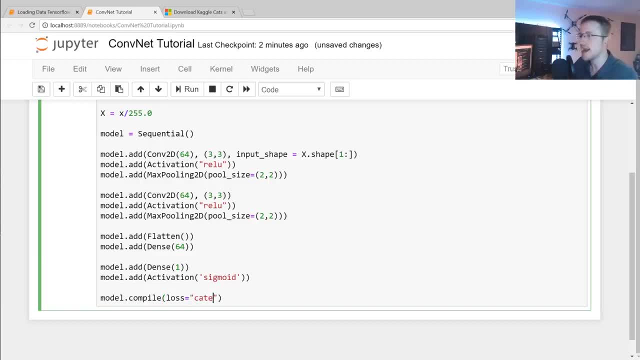 loss equals and we're going to use Categorical. Actually we'll use- so you could use cat, It's dogs and cats. so in this case We can use categorical or, I'm sorry, binary Cross-entropy- wow, how many times am I a trip over that? but you could use categorical and then optimizer in this case. 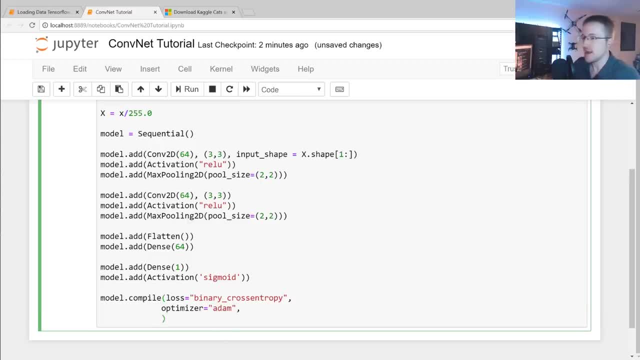 We're gonna go with Adam, because that's what we always go with, and then metrics equals accuracy. Now what we want to do is run the fitment. so we're just going to say: model that fits Xy. we can specify the batch size. This is how many at a time do we want to pass again? 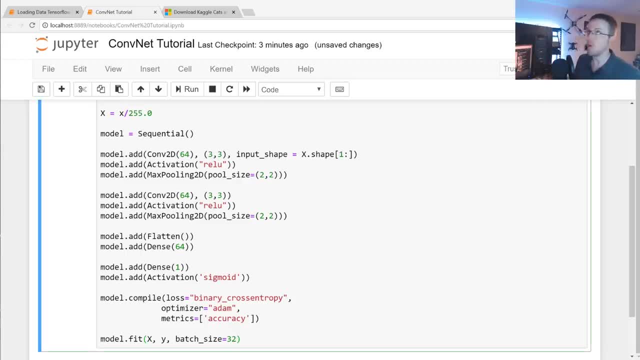 We've got 25,000 samples. you probably don't want to pass one at a time, But you also don't really want to pass all at the same time. It's generally a good idea to do something between like somewhere in the 20s to. 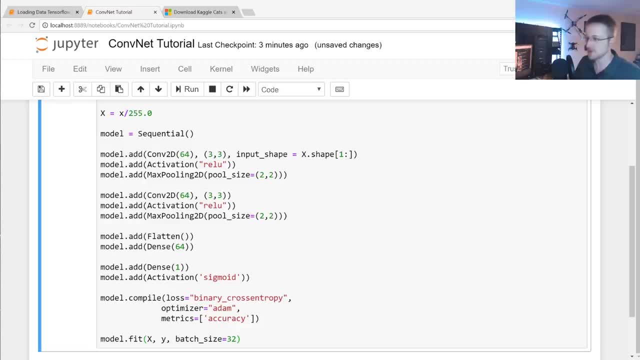 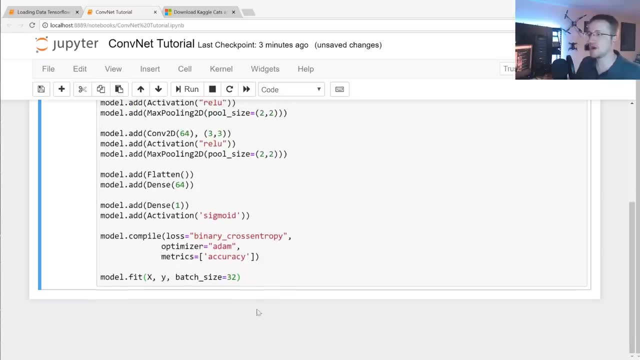 Maybe 200. usually I find negative results start coming in if I start trying to do like a batch size of like thousands. But it depends on the size of your data. So it's really gonna kind of scale with how big your data is. if you've got like a data set of a billion samples. 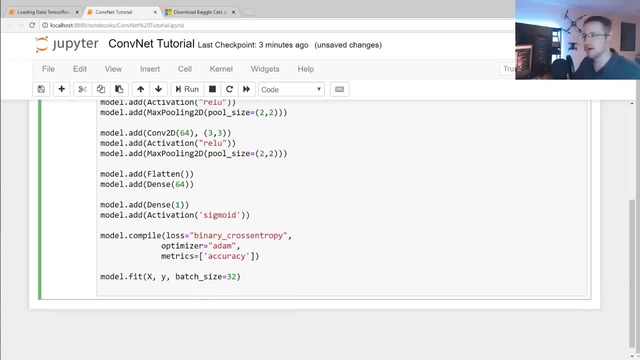 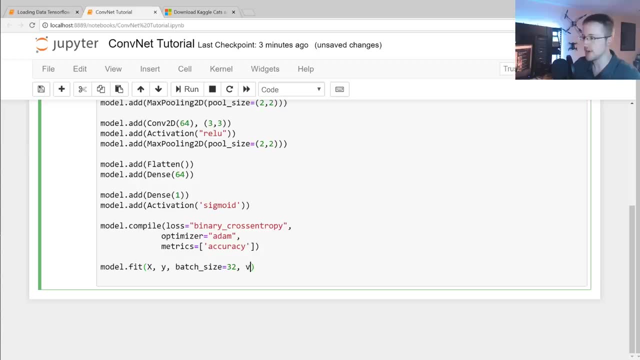 You could probably get away with a batch size of a few thousand, but anyways, yeah so model that fit batch size. We'll talk more on that in a little, in the next two. So, anyways, validation split. This is the kind of out-of-sample data. 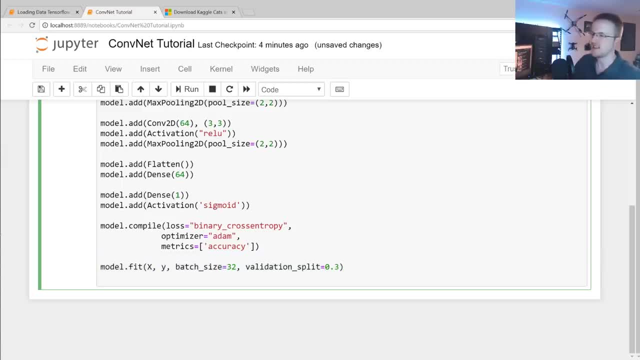 We're gonna say we're gonna save 30% and in fact That's a pretty high. Let's not do 30%, Let's just do 10%. So, model that fit 10% and great. so let's let's train the model, make sure we don't hit an error. 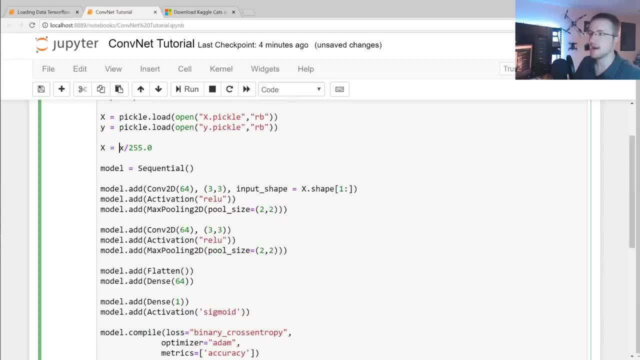 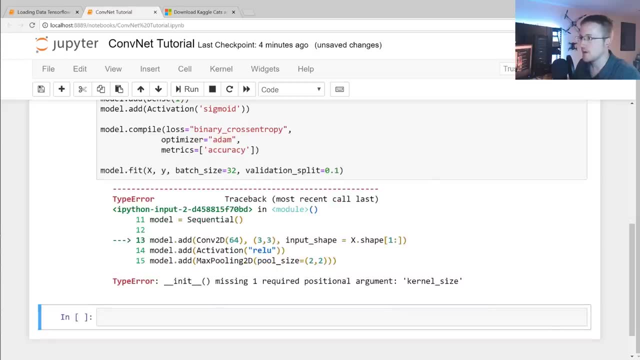 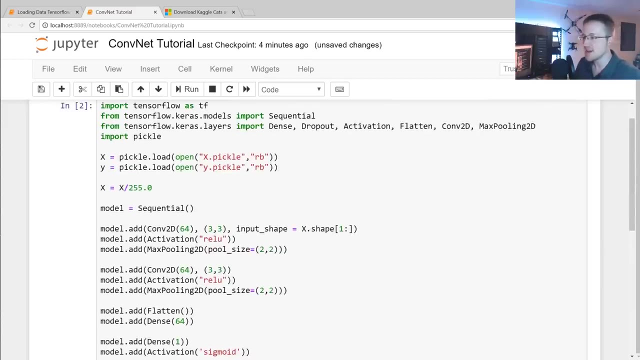 We did: X looks like a lowercase X. We need a uppercase the X. I Knew I felt weird there. Let's see one record kernel size, do. Okay, now I know what I've done. I knew I felt like I was like: wait, something's wrong here. 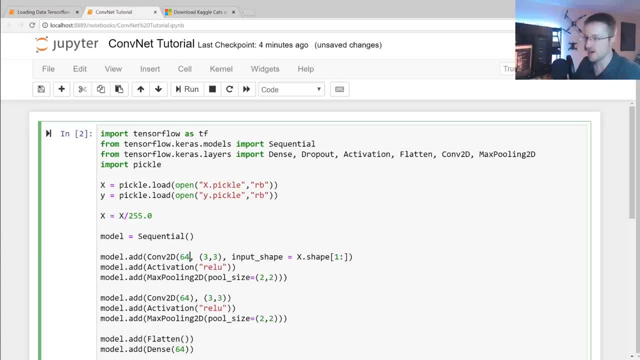 So I closed off with this 64 and we need to put it here so. so I Always get confused with why are you doing it. I would get confused when it comes time to do parentheses while I'm doing tutorials, so let me just space everything out real nicely. 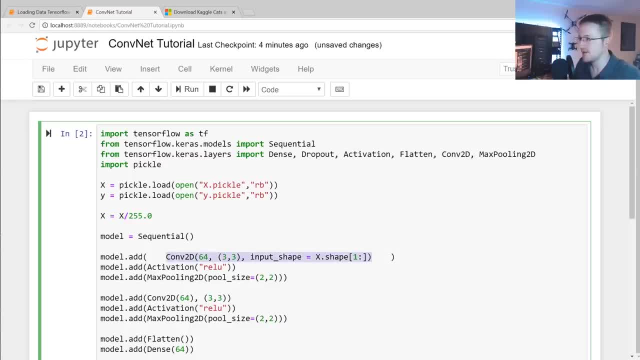 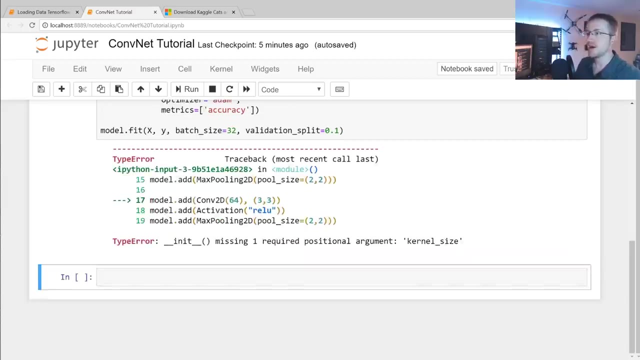 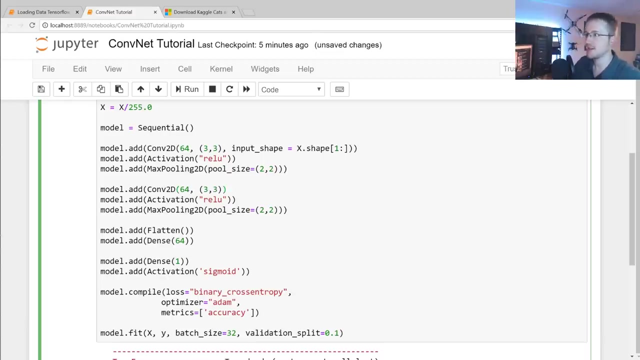 So this is the conv layer- right, it's 64 units- followed by the next parameter, which is the- the window size- followed by the next parameter, which is the input shape. Okay, oh my gosh how many. oh, We did it because we copy and pasted, got it, chickity check. 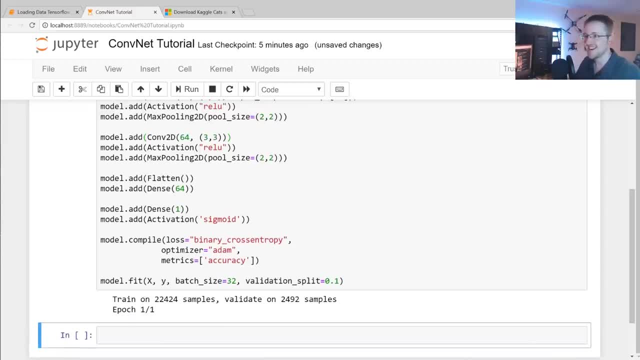 Please, no more errors. They'd be really nice. All right, so I think we're training finally, yes, all right, So we're already at 64- 65. We're doing pretty good. I Don't know if we said, oh, we didn't specify epochs, so let's go ahead and specify, so, even after one. 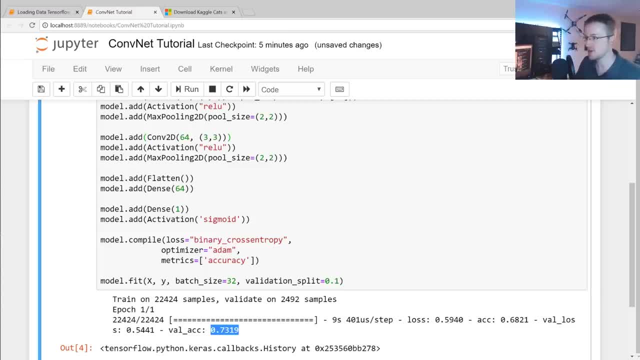 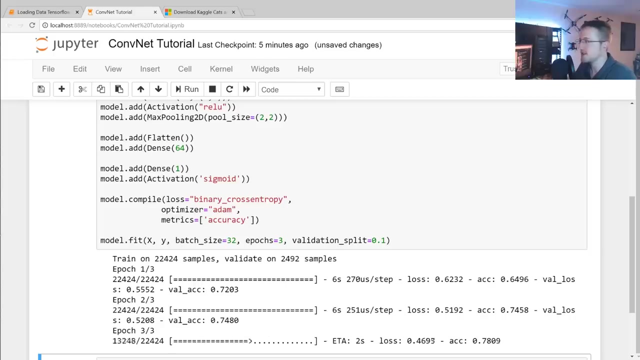 We got a 73 percent validation accuracy, which is pretty good, So let's go ahead and pass in one more epochs equals three. Let's do it a few more epochs of this data, Even better than the last one. Okay, so that's looking pretty good. We were up to 74- 78. looks like we're gonna Maybe breach 80. 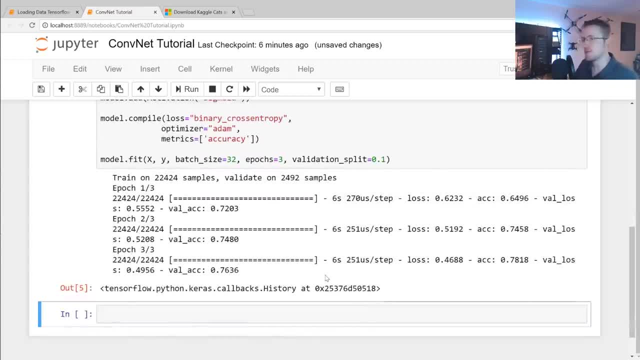 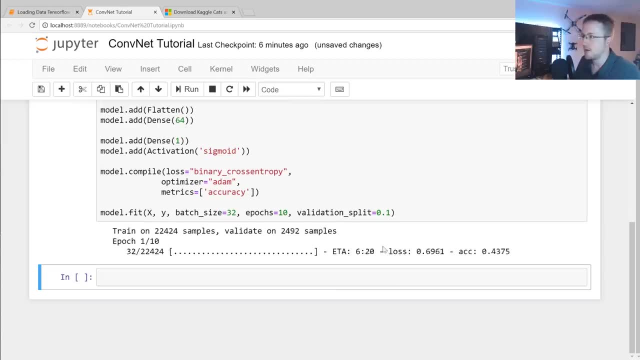 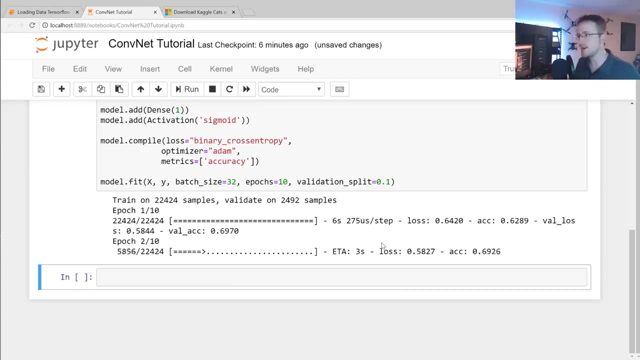 We'll see, not yet anyway, but if we kept training this, probably for like 10 epochs or something like that- In fact I'll plug in 10 for the rest of my talking here- Chances are we'll probably breach 80, which is pretty good because that means we're classifying cats and dogs pretty darn accurately. 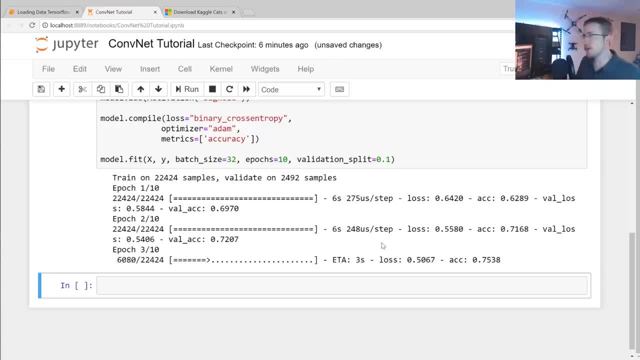 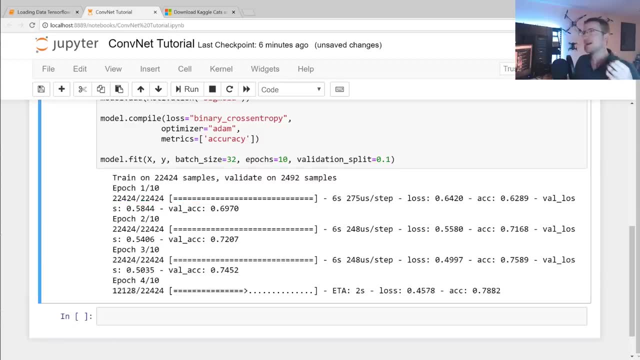 so in the next tutorial, What we're going to talk about is: okay, How do we read these numbers? like what it? you know, how do we actually read laws? How do we measure? you know how we like read the accuracy and especially like: what about accuracy versus? 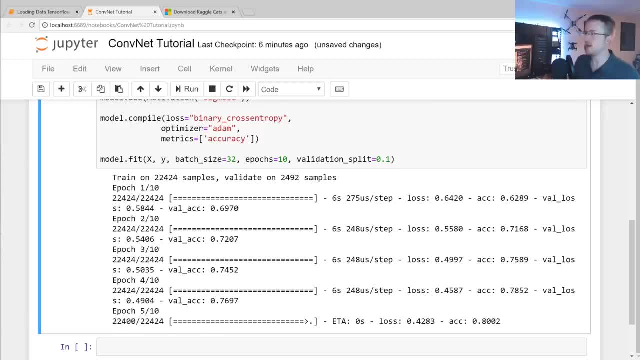 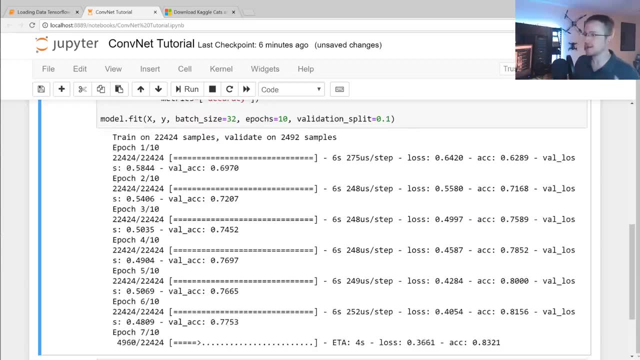 Validation accuracy, like in this case, is kind of wonky. we got a better validation, accuracy over accuracy- It's kind of weird, and we did it again. This is the first time we didn't, so I'll talk about like little stuff like that. That should be kind of red flags. at least initially It's not that big of a deal, but if your model consistently does that, that's a problem. 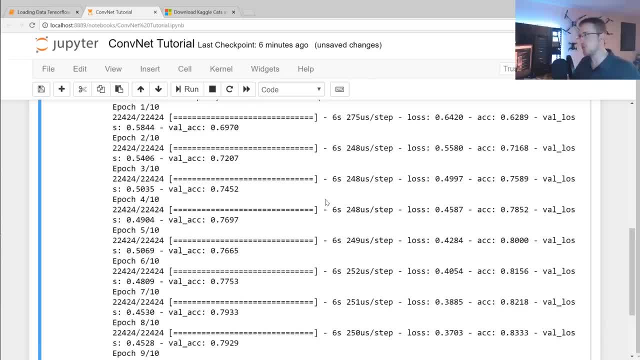 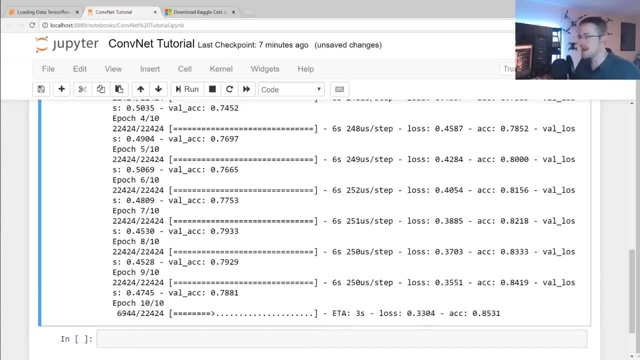 So we'll talk about some of the patterns that you should start seeing and that you should watch out for as you begin to train models. so, Anyways, that's all for now. If you've got questions, comments, concerns Whatever, you can feel free to leave them below if you like this content. 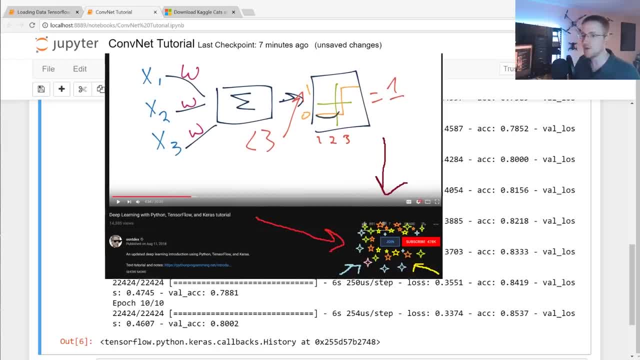 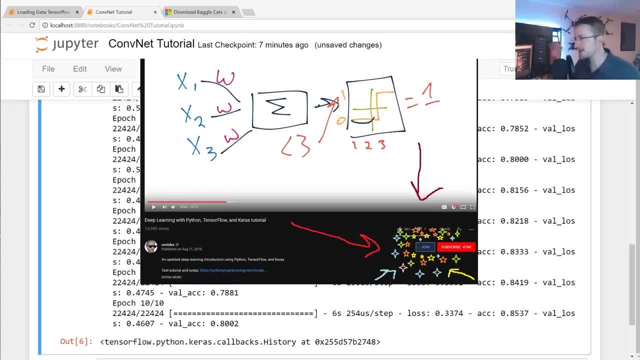 You can support the content by clicking on that beautiful join button right down there. if you join, it helps support me in the channel. Also, you get various perks, like a little Badge next to your name. you also get early access to videos- just like this one- and also shout out from time to time when people 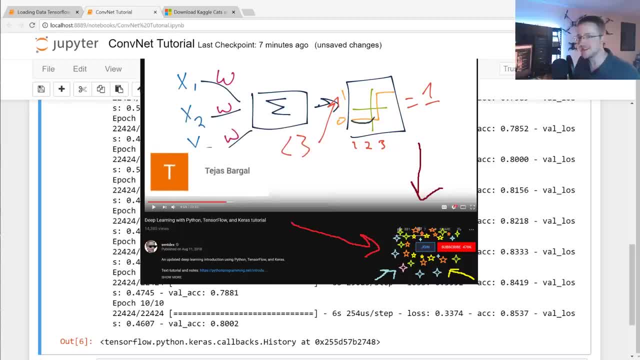 Join, so my most recent member is Tejas. Thank you very much for your support. good sir, You help support my mug addiction. okay, so that's it for now. in the next tutorial, We're going to be talking all about tensor board, which is absolutely essential for